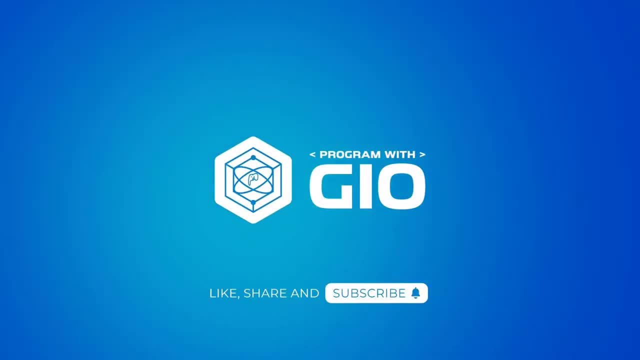 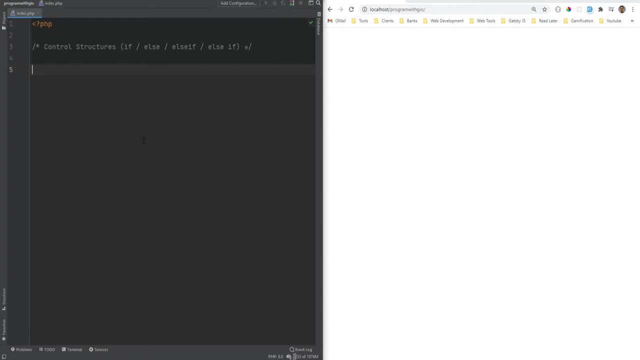 A PHP script is made of series of statements where a statement can be an assignment, a function, call, a loop, if else, conditionals and so on. As you know, in PHP statements end with a semicolon and you're able to group multiple statements within curly braces. A control structure is something. 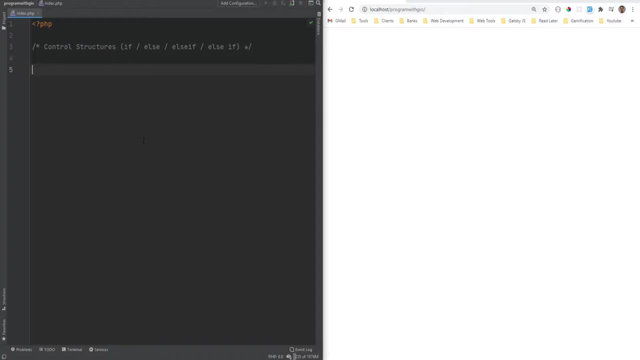 that allows you to group multiple statements and also allows you to control the flow of the code execution. You could, for example, execute A only if condition B passes or keep executing A until condition B is met. The first control structure that we're going to cover is the if conditional. 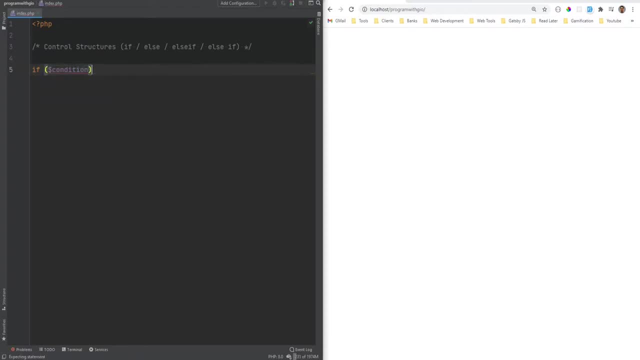 statements. The syntax is if some kind of condition and then curly braces, and within the curly braces you put the blocks of code or statements that you want to execute only if the condition evaluates to true And this condition here basically can be any kind of expression. It could be as simple as 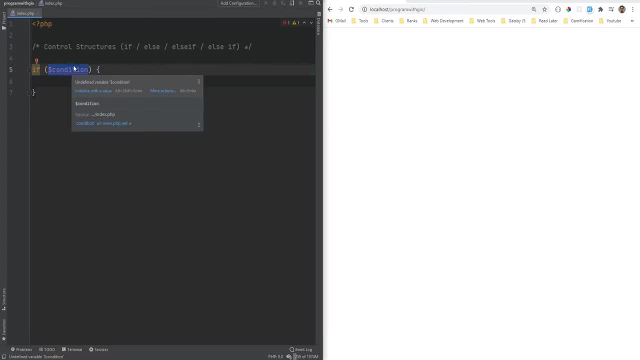 just a variable like this, or it could be as complex as using multiple operators, including the logical operators and so on. So, for example, let's implement a simple gradient. So let's say score is 95, and then we can do: if score is greater than or equal to 90, echo A. If we 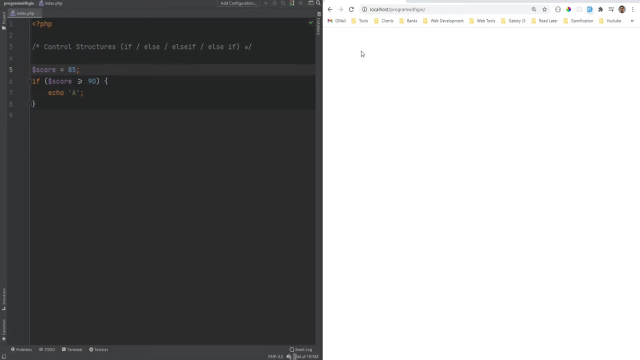 refresh, we get A. If we change this to 85, now it prints nothing. So, as you can see, this statement executes only if this evaluates to true. Now for simple statements like this: when you have one line, you could actually remove the curly braces and it will still work. If we refresh, nothing is. 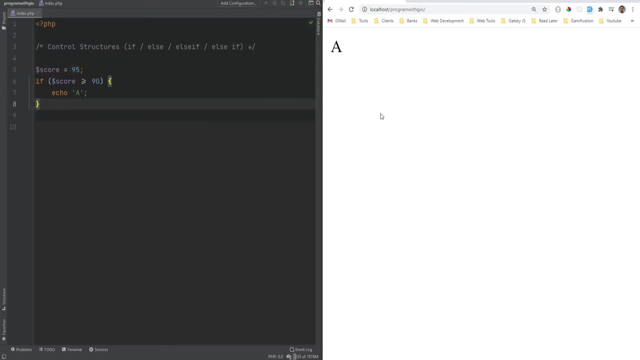 printed. If we change this back to 95, it will print A again. I personally recommend to always do this, because it makes code more readable. So what happens when the condition fails? What you can do is, if the condition fails, you could execute a default block of code, and that is by. 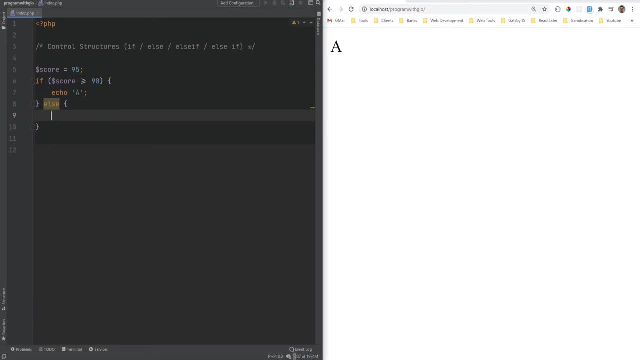 using the else case here, So you could do else. and within the curly braces you put the block of code that you want to execute in the condition when this expression does not evaluate to true. So here you could say echo F. So if we refresh we're getting A, but if we change to 85, we're. 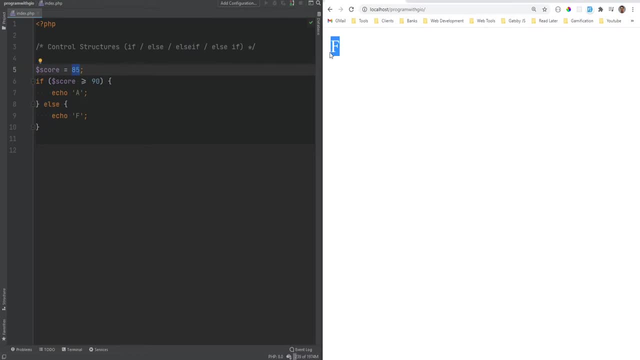 getting F, But that's pretty harsh right, Because if you have score 85, you would never get F. This actually need multiple conditions, and you can do that by using else. if So, we could do else. if score is greater than or equal to 80, echo B, and then let's do the same for the C and D grades. So 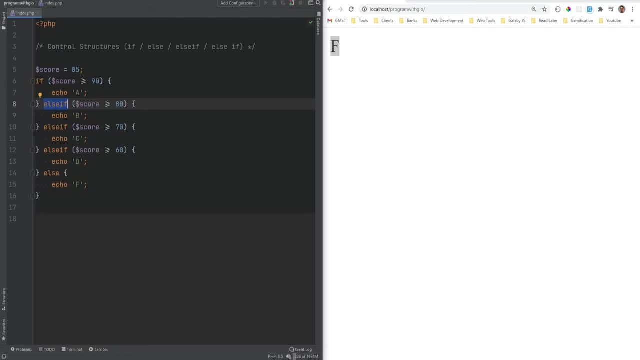 as you can see, you could chain as many else if conditionals as you need. So in this case, since it's 85, we're going to get B. If we change this to 65, we're going to get D, And if we change 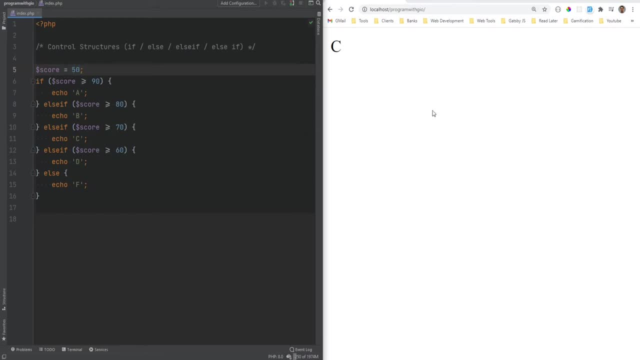 this to 75, we'll get C, And finally, if we set to something like 50, we'll get F. Now, the other way of doing else if is by using space here, and this will work exactly the same way. So if we 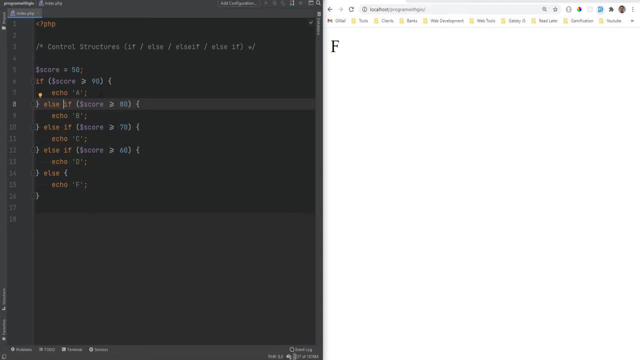 there is a syntactic difference between the two, but when you're using the alternative syntax, which I'm going to talk about in a minute within the HTML, you need to use the one without the space. I personally always use the one without the space. You could also nest as many if else. 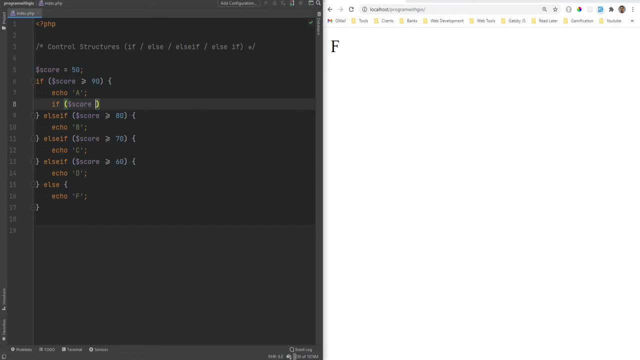 conditionals as you want. So you can here. you could say: if score is greater than or equal to 95, echo plus. So that way, if you get something like 95 or 96, it will print out A plus. So 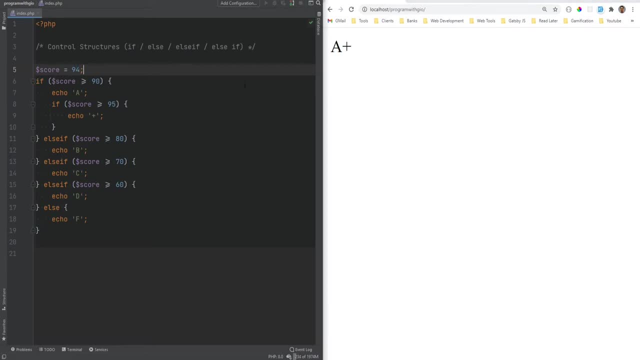 if we set this to 95, we'll get A plus. If we set to 95, we'll get A plus. If we set to 95, we get A. And same goes for the other cases. You could nest it within the else ifs and you could. 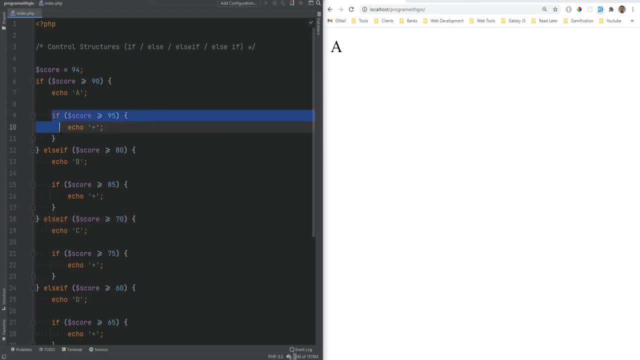 nest it within the else as well. So, as you can see, we're repeating a lot of the code here and don't worry about that right now. We'll cover about the best practices and how to avoid code repetition in the later videos. So if we change this to 76, we'll get C plus If we change it to. 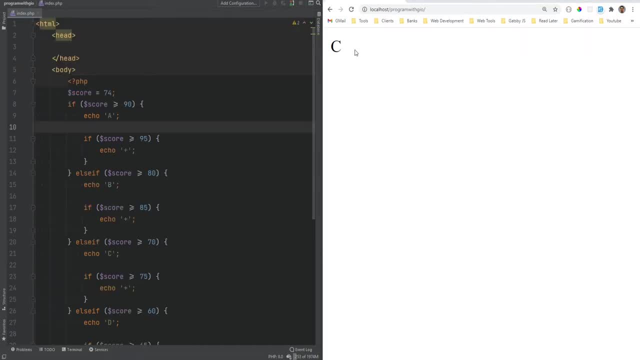 74, we'll get just C. So let's embed this within the HTML and go over the alternative syntax. But this kind of looks ugly right, Because we're embedding a lot of PHP within HTML. Also, what if we wanted to print some kind of styling, or print some kind of HTML elements with 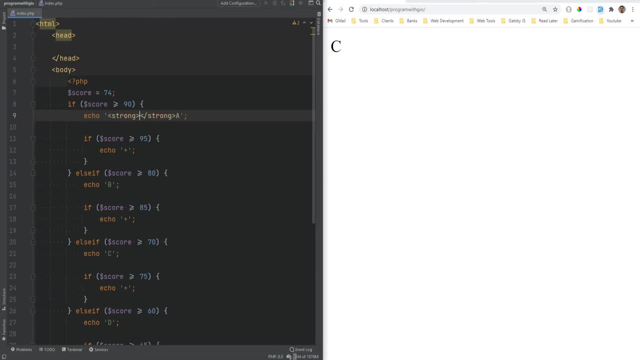 our values. We could, of course, echo out the HTML directly like this, but then that also does not look readable. Let me remove these additional if statements from here, so that we have less code to work with. We could do something like close the PHP tag here and then remove the echo from here.